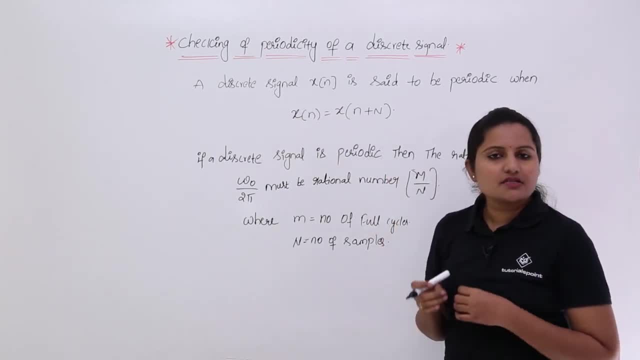 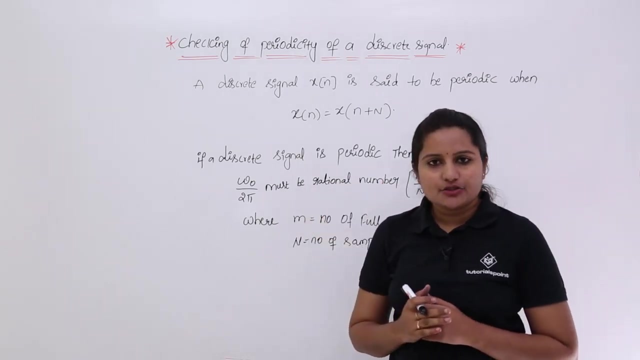 x of n is equivalent to x of n plus capital N. This is very similar to continuous signal periodicity condition. So for n for every n time interval the signal need to repeat. Then that is said to be periodic. So now, if a discrete signal is said to be periodic, 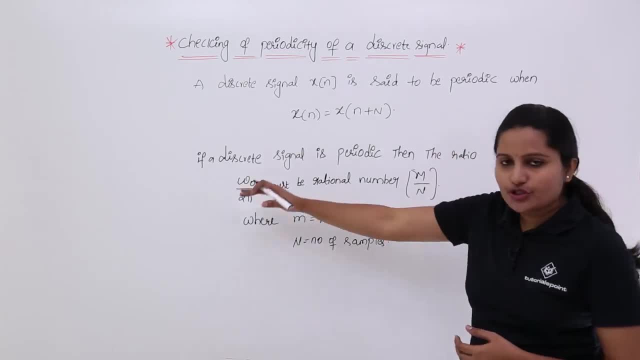 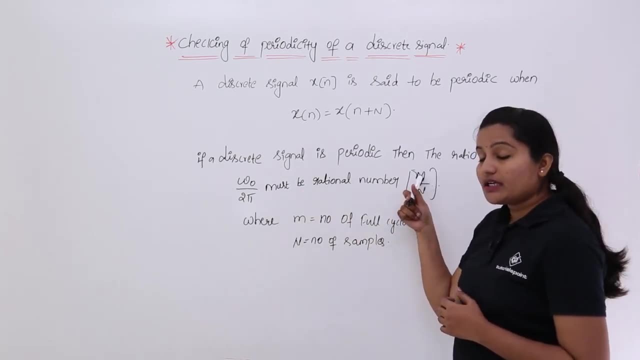 if a discrete signal is periodic, then the ratio of its fundamental frequency divided by 2 pi must be a rational number. That means that is equivalent to m by n, where m is equivalent to number of full cycles in the original continuous signal and where capital N, that means denominator. 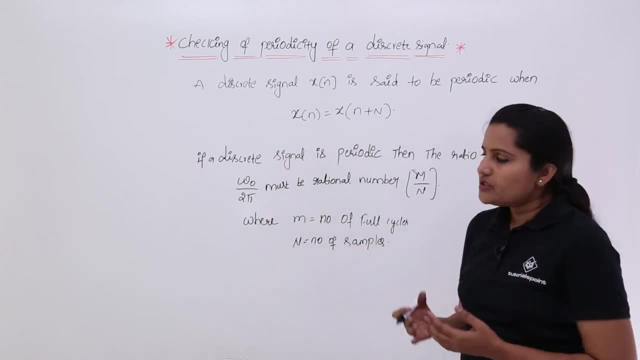 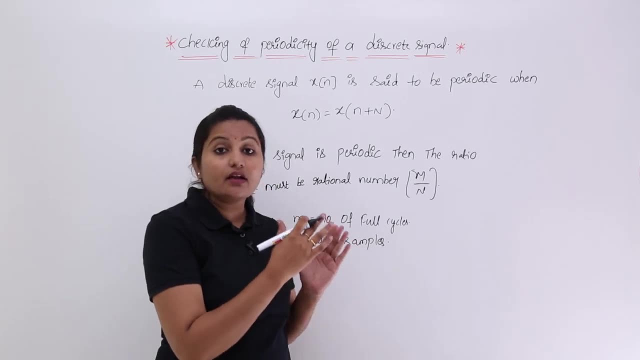 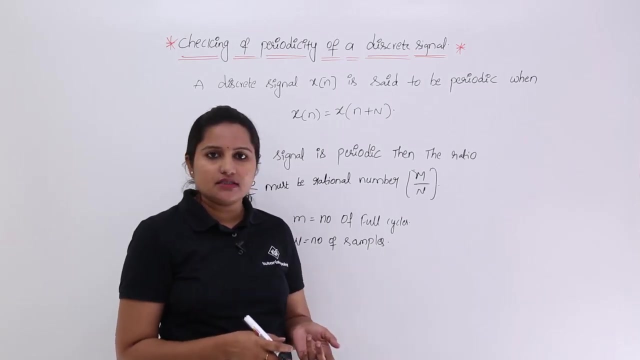 in this ratio will become number of samples. So, coming to checking of periodicity of discrete time signals, coming to continuous time signal, I want to compare these two. So when a continuous time signal is given, we are having two methods there. I discussed this. 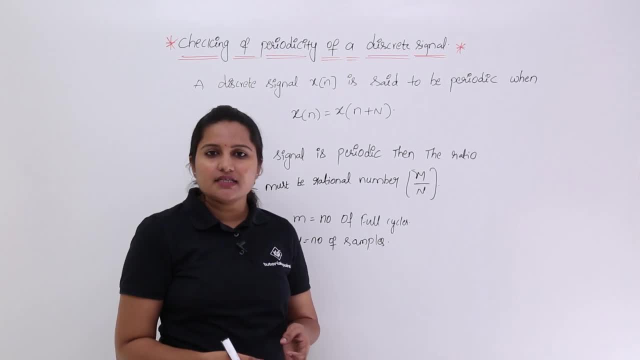 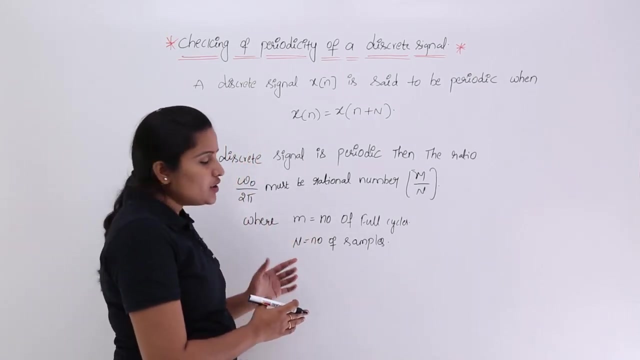 two method. one is GCD method. another method is T1 by T2, considering the ratio of time periods, Ratio of time periods methods and GCD methods. we are having, for continuous time, signal periodicity check. for discrete signals, To check periodicity, we are having an equation, omega, not by 2 pi, this must be a rational number. 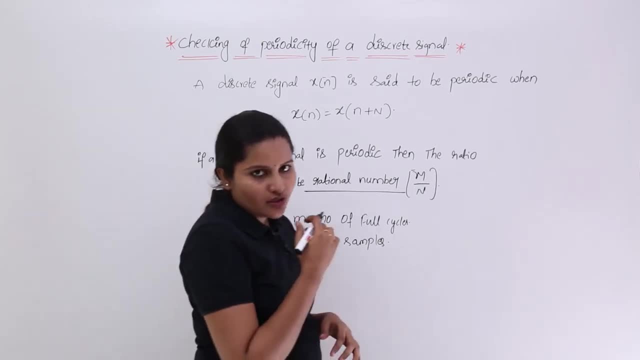 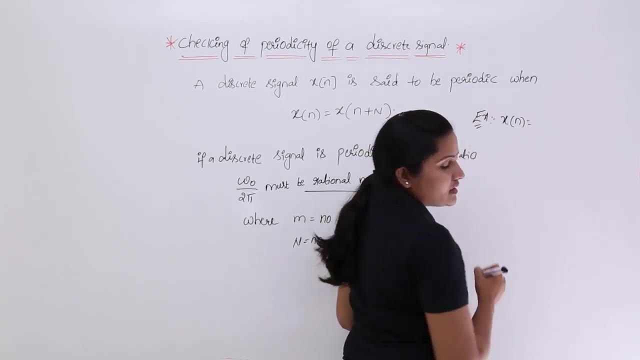 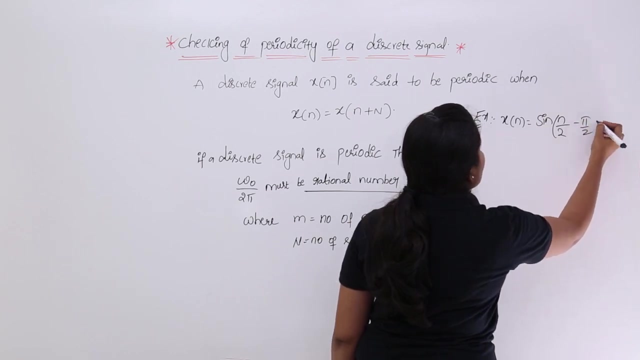 that means integer by integer. So now I am going to consider some examples. So they given example, for example, they given, like this example: x of n is equivalent to. you are having sine n by 2 minus pi by 2. like this, they given x of n is equivalent to sine n by 2 minus pi by 2.. So you 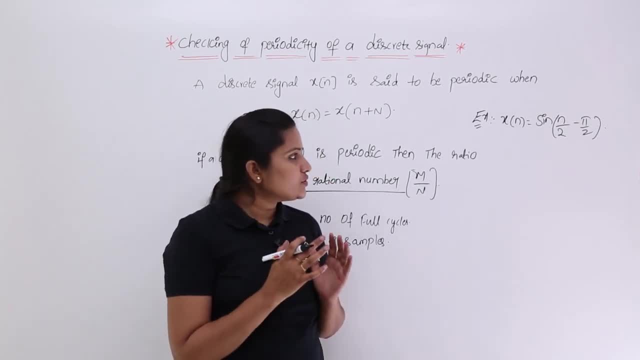 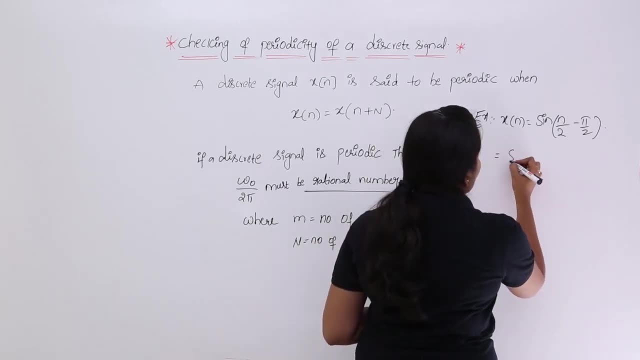 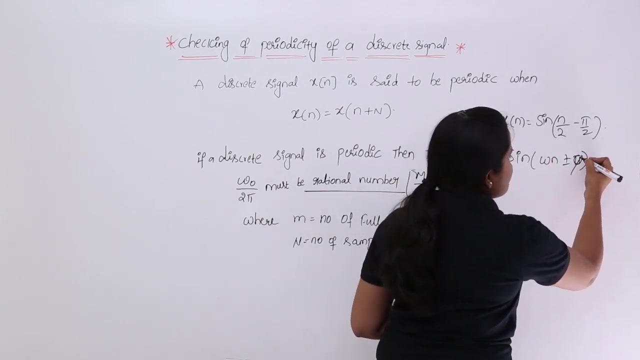 check whether the signal is periodic or not. So to check this, I want to compare with the basic definition of sinusoid. So that is, I want to compare with sin. omega n plus r minus phi. I want to compare with or phi. this is phase. So here this is discrete sinusoid where omega is. 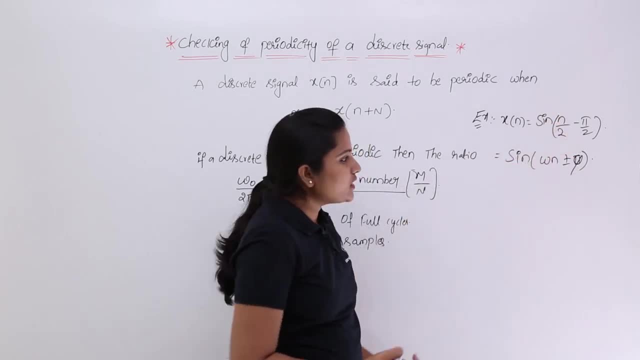 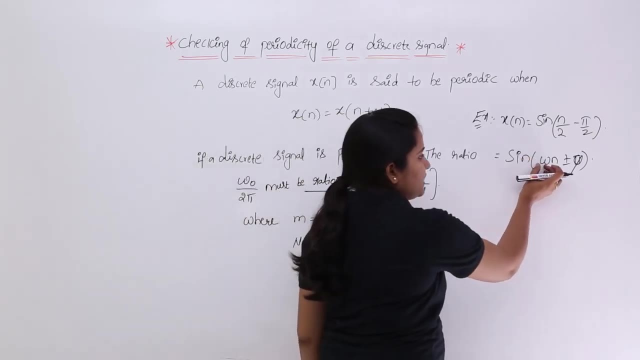 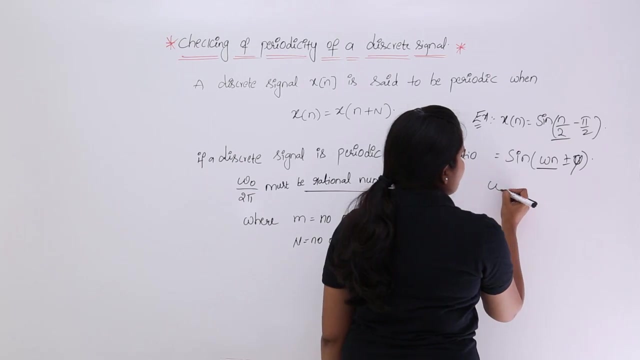 equivalent to omega. n is equivalent to n by 2.. So if you compare these two, we do not require any phase value to calculate periodicity of a signal. we just need this omega. whatever angular frequency is there that only we need. So if you compare these two, I am going to get my omega is. 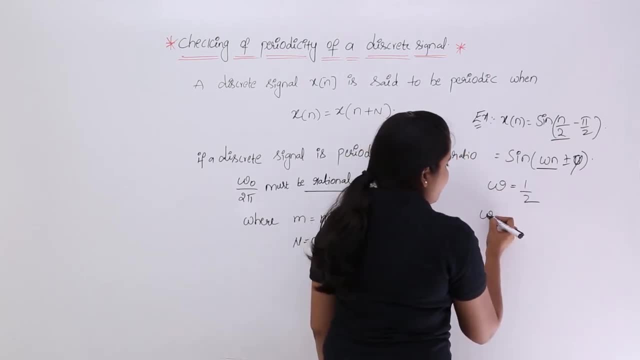 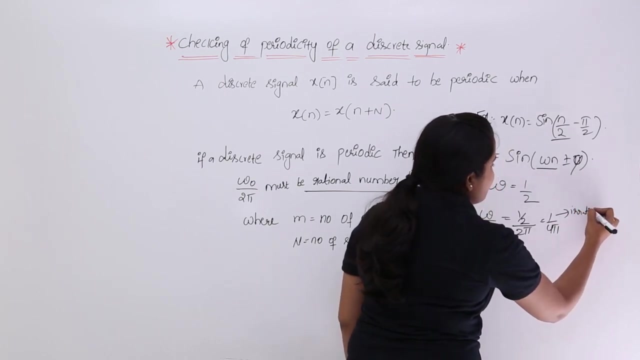 equivalent to 1 by 2.. If you calculate omega by 2 pi value, or omega naught by 2 pi value, then what you are going to get is 1 by 2 by 2.. That is equivalent to 1 by 4 pi. This is not rational number, this is irrational number, and 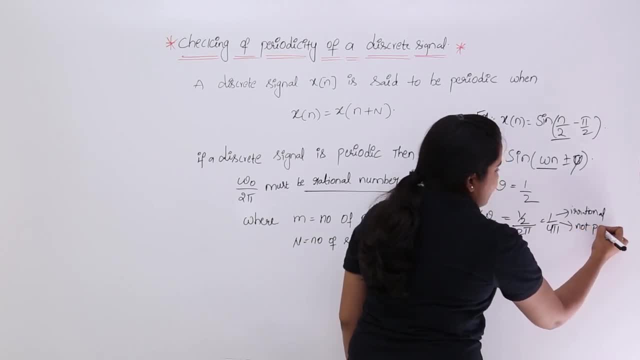 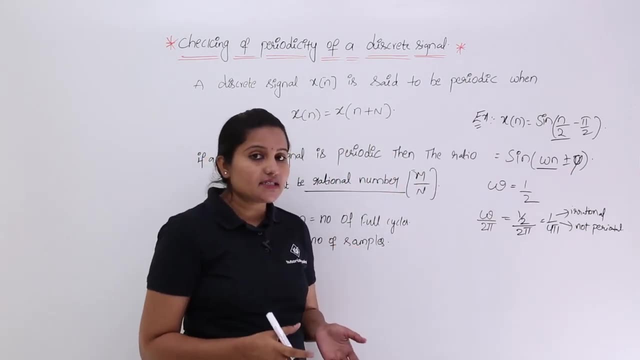 it is not periodic signal, not periodic. Why? Because this is a irrational number. that is why this is not periodic. So, like this, we need to check periodicity of discrete signals, For discrete signals do not apply that GCD concept and other. t 1 by t 2, that means ratio. 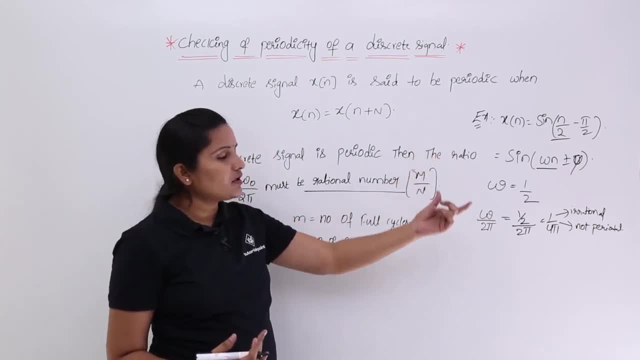 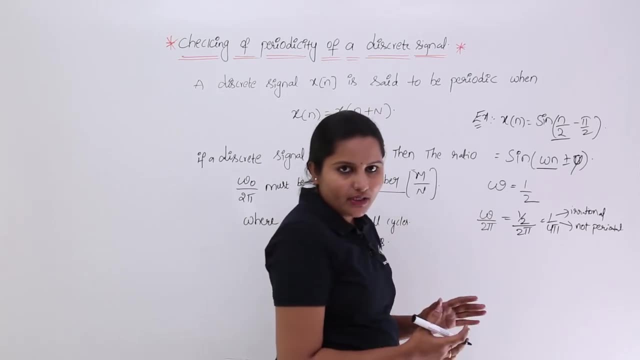 of time periods concept. You need to apply this concept for calculating periodicity of a signal. So, like this, we need to check periodicity of discrete signals. So now, for example, I am going to consider another example. So here, for example, x of n is: 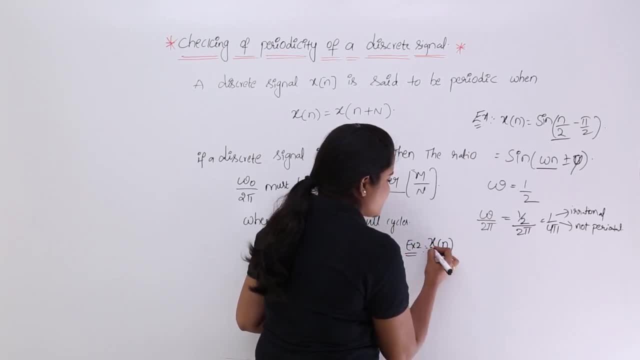 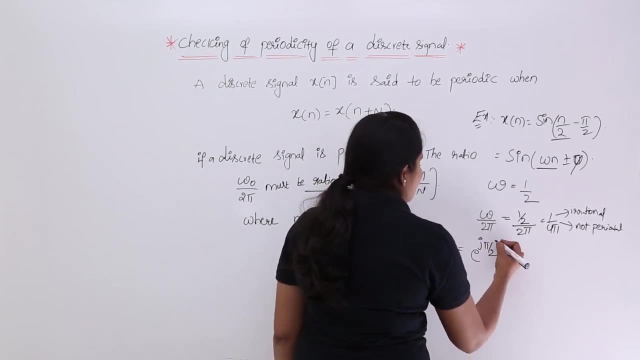 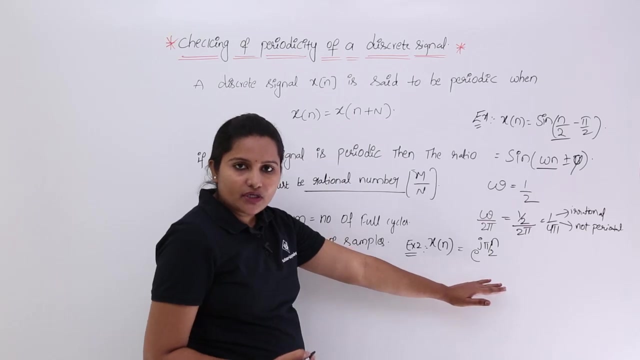 equivalent to this is example 2. I am going to consider for discrete signal periodicity. So x of n is equivalent to e power, j, pi by 2, n, For example. if you are having like this, So this is a signal given, Then if you need to check this is a periodic or not, then you 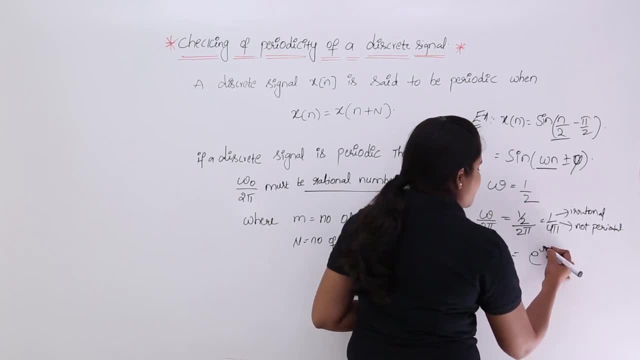 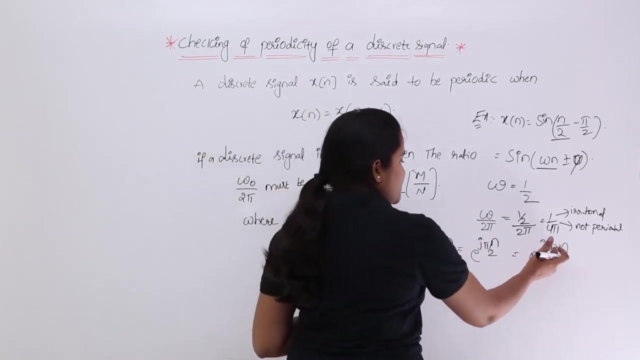 need to compare with basic exponential j omega n, as this is discrete signal. you need to compare with j omega n. that is a positive exponential e power j omega n. If you compare these two, then omega will be equivalent to pi by 2.. If omega is equivalent to pi by 2, 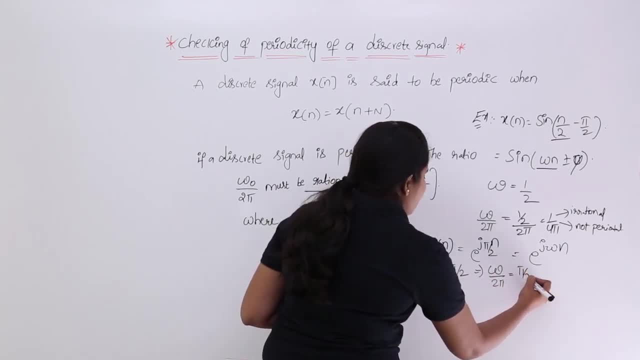 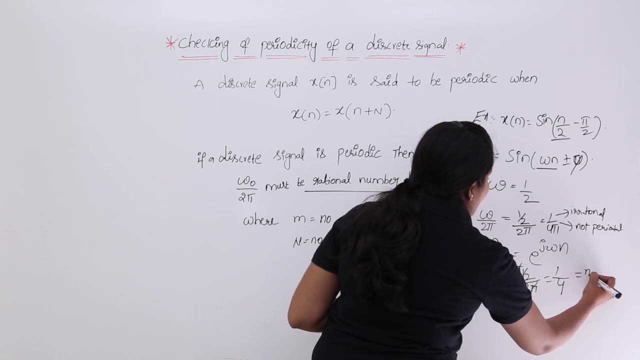 this is equivalent to pi by 2. omega by 2 pi will become pi by 2 by 2 pi. Then you are are going to get pi. pi will be cancelled. then this is equivalent to 1 by 4. now your m by n value is: 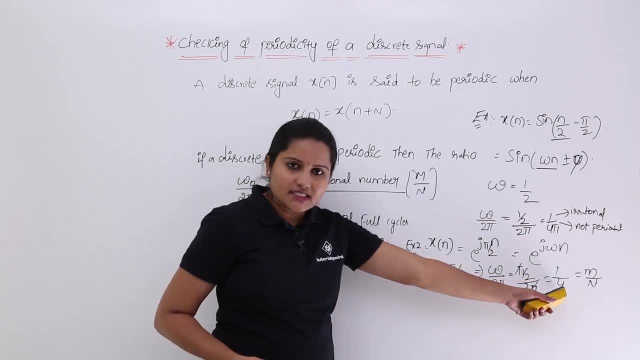 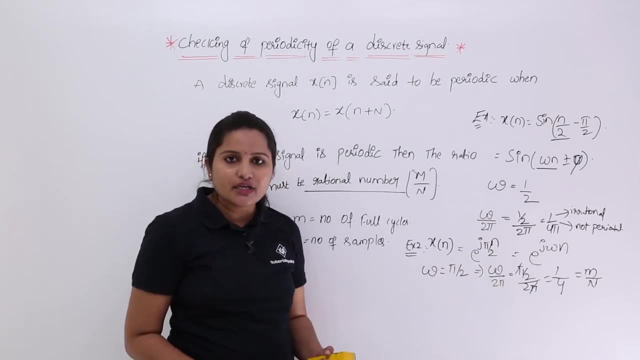 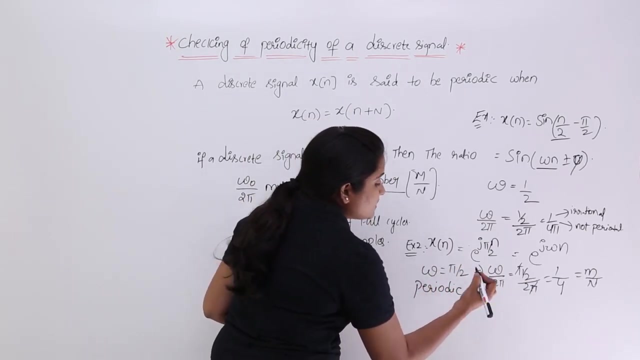 equivalent to 1 by 4.. So this is in integer by integer format. your ratio of m by n is equivalent to integer by integer or rational number. So definitely you can say this signal is a periodic signal, periodic signal always. your period of discrete signal will be samples, number of samples.